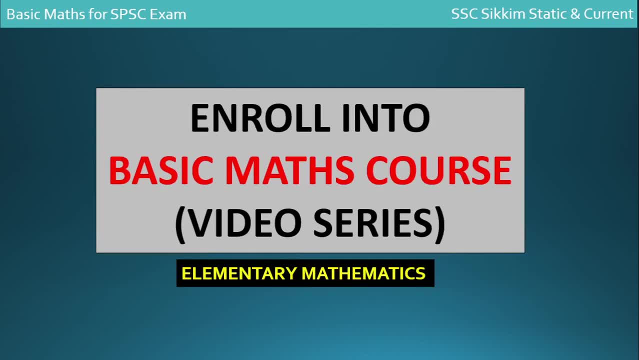 So for that you can just see the description box. So let's proceed. But before moving you can just enroll into basic maths course. We have launched a basic maths course in SSC, Sikkim, In SPSC, as much as you can. 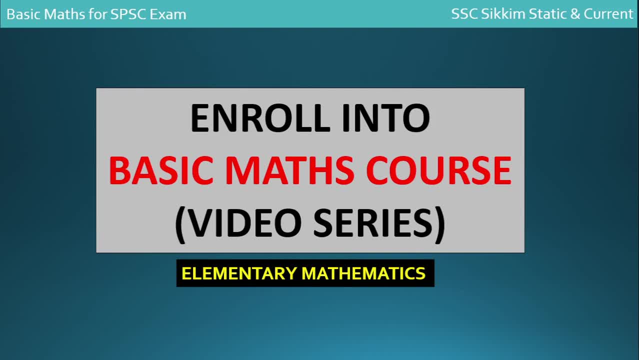 We will ask you basic maths questions. In that you will get the videos topic-wise. We have also discussed the previous questions, So you can just enroll into it. It is a 3-4 hour session. There are 12-13 videos. 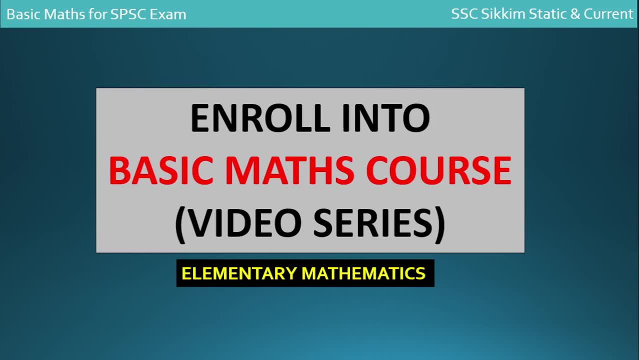 We will cover them in 3-4 hours And then you will have a gross idea on what kind of basic maths questions can be asked and what concepts are involved in this, So you can just enroll. Details are in the description. 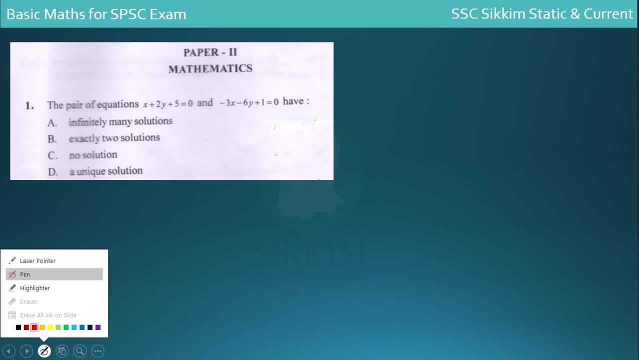 So let's proceed. First question: You are going to see this question. It is a question from linear equation in two variables. It is from class 10.. Here we have seen two equations And we are going to see what kind of solution it has. 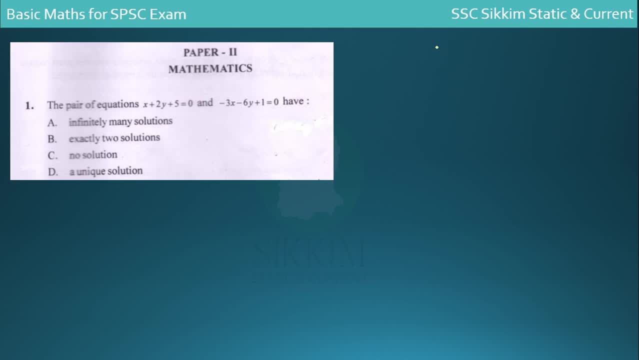 For this you need to understand a concept. You have already studied it in class 10.. What is that concept? First of all, what is the general form of linear equation, General form of linear equation in two variables. Now we will write two equations together. 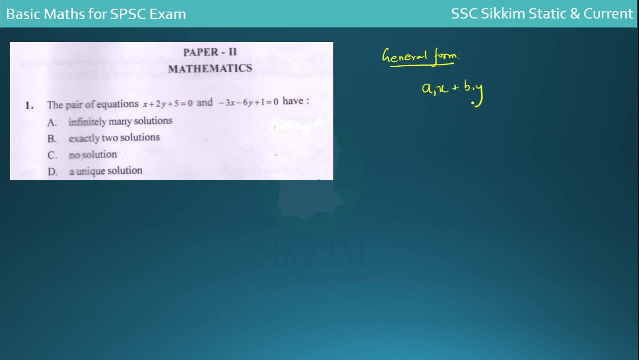 First one is: a1x plus b1y Plus b1y plus c1 equals to 0.. Now we will write: a2x plus b2y plus c2 equals to 0. with another equation Now: a1, b1, a2, b2 cannot be 0. 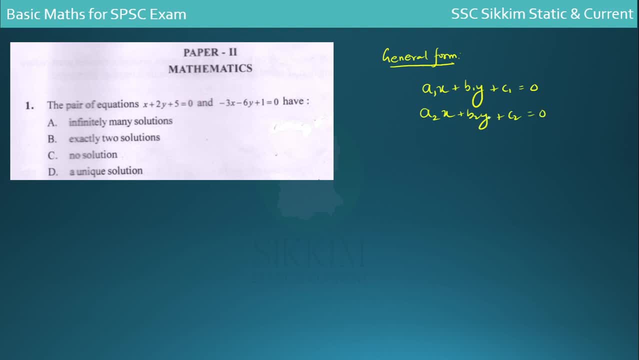 Because 0 is converted in one variable, So 0 cannot be 0.. c1, c2 cannot be 0.. Now let's see this form. In this form we will look at the ratio of coefficients. What is the ratio of coefficients? 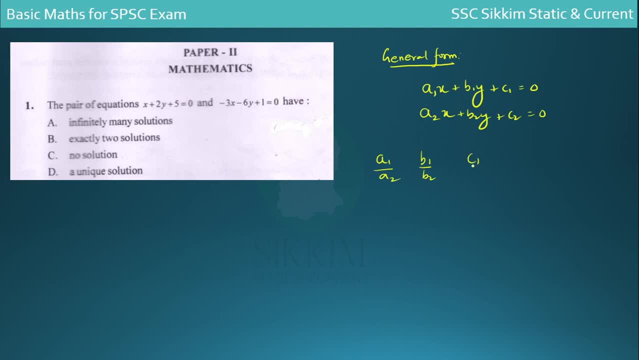 a1 by a2.. b1 by b2. And c1 by b2.. c1 by c2.. Now we will look at the ratio of coefficients to know the solution. Now there are three conditions: First, second and third. 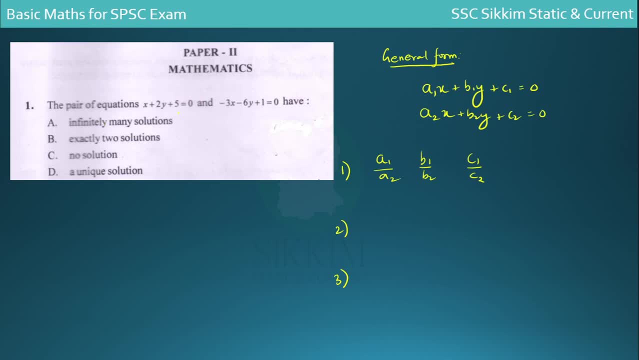 In this equation, you can see that there are infinitely many solutions. That means: there are many solutions. There are no solutions. There are unique solutions. There are no solutions. There is only one solution. There are many solutions. Now, there are exactly two solutions. 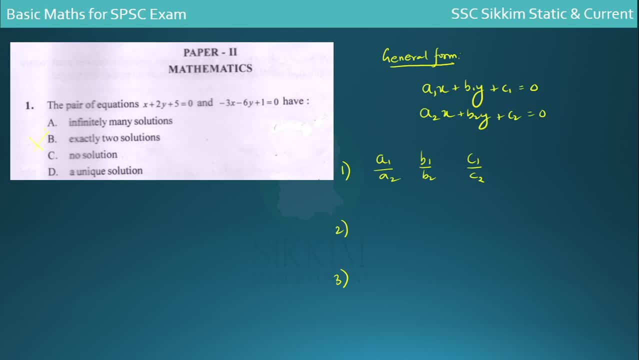 Option B will be discarded. So our answer is A, C and D. Now let's see: a1 by a2.. b1 by b2.. c1 by c2.. Now if in this coefficient the first ratio is not equal to a1 by a2.. 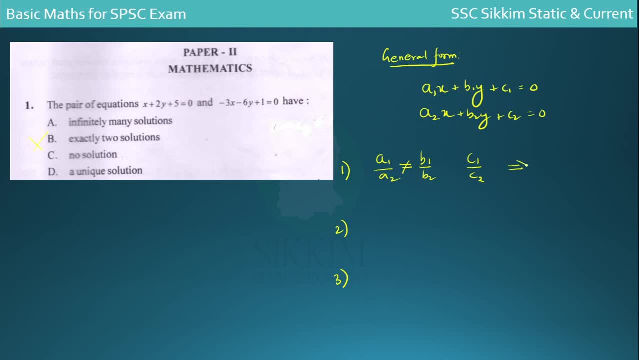 That is, a1 by a2 is not equal to b1 by b2.. We do not have to check c1 by c2.. In this case our solution is unique. That means the value of extra y is only one. 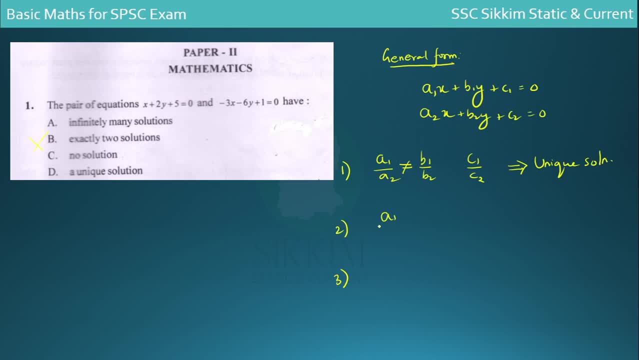 Do you understand? Now, in the second case, if a1 by a2 and b1 by b2 are equal And c1 by c2 are also equal, The ratio of coefficients, The ratio of three coefficients, is equal. In this case, there will be infinitely many solutions. 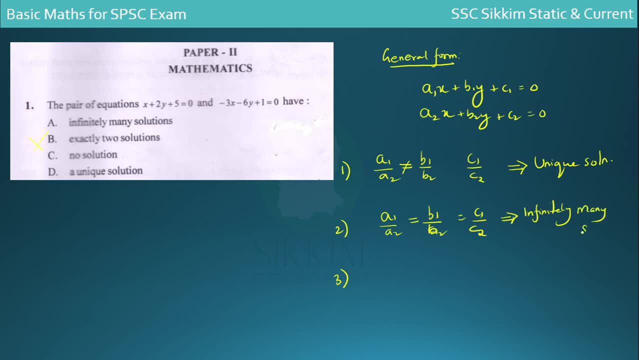 Okay, Infinitely many solutions. Now the third condition is: a1 by a2- is there? b1 by b2- is there? Now, these two are equal. The first two ratios are equal, But the third is not equal. 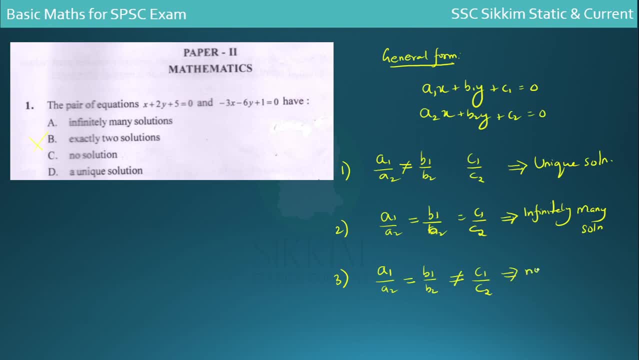 c1 by c2 is not equal. That means at that time there will be no solution. There will be no solution, Do you understand? So we have to check these three conditions. Now the first equation. You can ask like this: 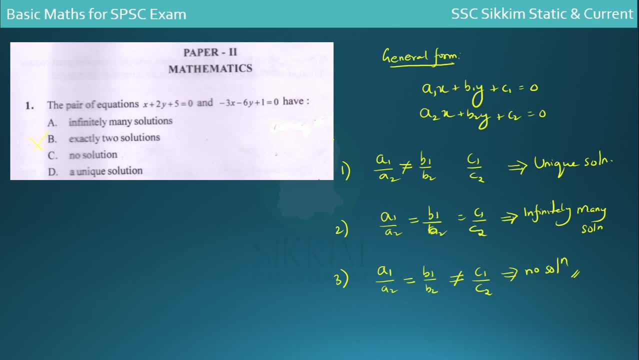 Does the pair of equations, this and this, have? what kind of graph? Is it an intersecting graph? Are the lines intersecting in the graph, Or is it parallel, Or is it coincident? You can ask like this. So at that time you have to understand the graph. 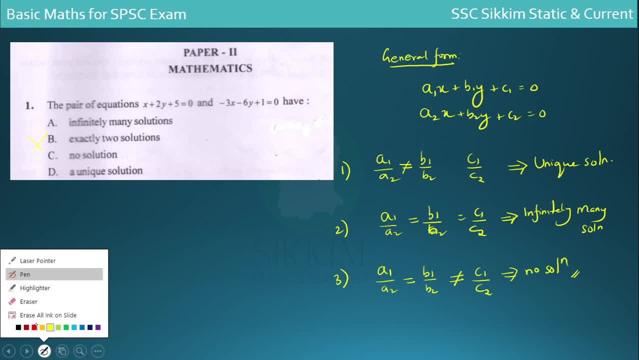 What is your graph in the unique solution? This is your revision In the unique solution. In the unique solution, the graph of the two equations is in a line In the Cartesian plane, in the coordinate axis. you have to plot the graph. 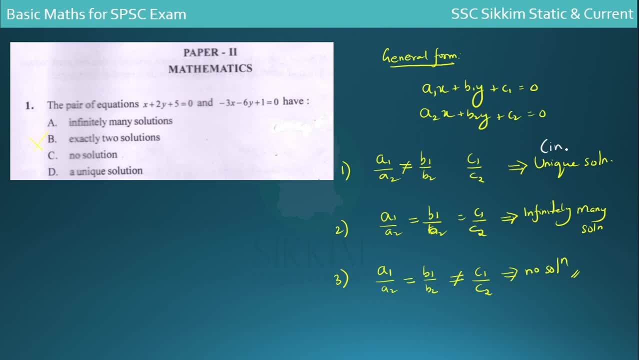 The graph is in that line. So, at that time, what is the unique solution? There are two lines in the two equations. What are those two lines? They are intersecting, Do you understand? And what is the infinitely many solution? 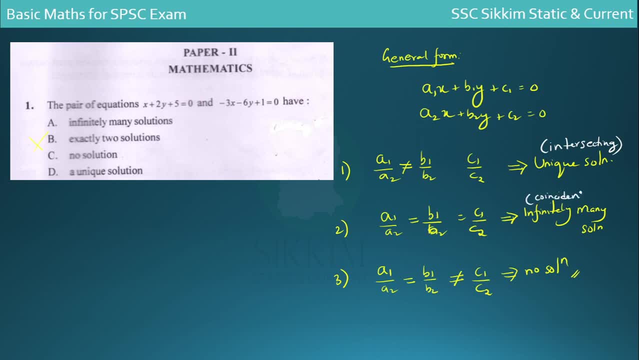 It is coincident, Coincident. Coincident means that two lines are intersecting at one place. Okay, And what is the no solution in the graph? It is a parallel graph. Okay, So parallel means no solution. Coincident means infinitely many solution. 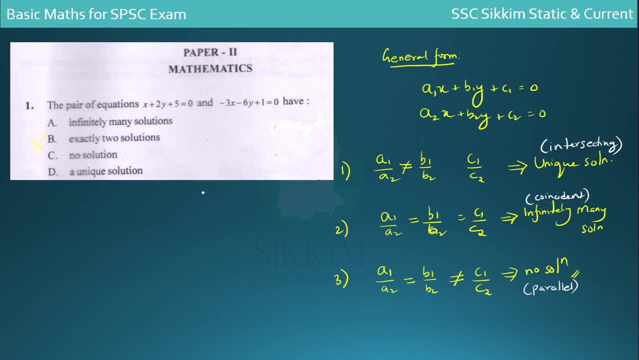 Intersecting means unique solution. Now let's solve this question. The pair of equation x plus 2y plus 5 equals to 0.. Minus 3x minus 6y plus 1 is equal to 0.. What happens? 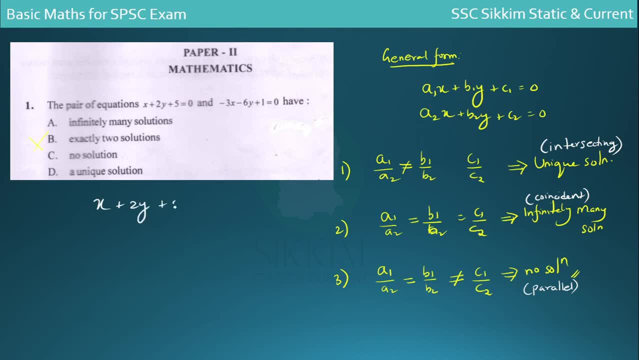 So let's write the equation first: x plus 2y plus 5 equals to 0.. This is the first equation. Minus 3x minus 6y, Minus 3x minus 6y plus 1 equals to 0.. 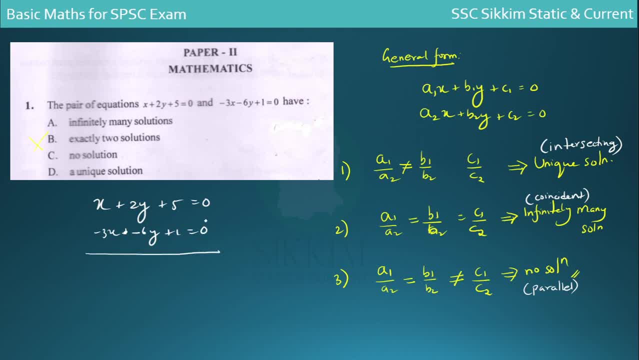 Remember this: This has to be equal to 0. If it is not equal to 0, then you have to take the term from above and make it equal to 0.. Okay, So this is equal to 0.. So after that, what will we do? 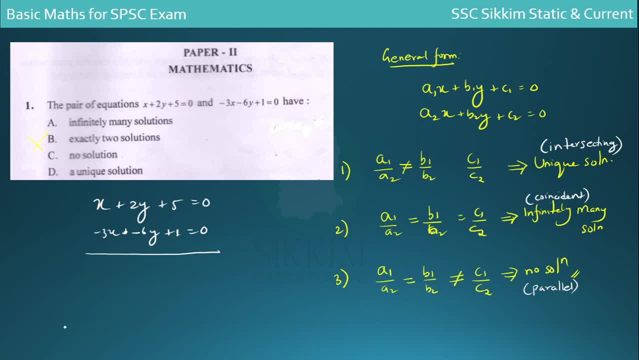 We will compare the coefficients. So look here: What is a1 by a2?? What is a1 by a2?? The upper coefficient of x is 1.. The lower coefficient of x is minus 3.. So we don't have to cut this. 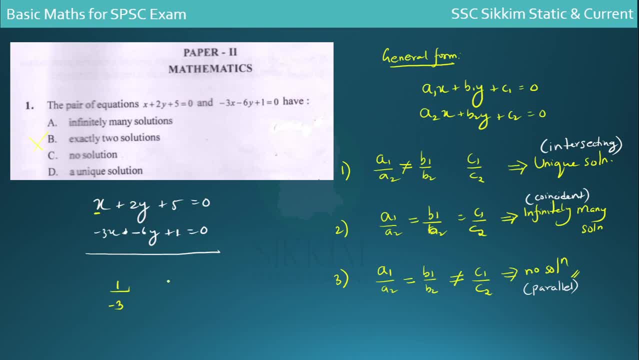 So minus 1 by 3.. Now what will be b1 by b2?? The upper coefficient is 2 and the lower coefficient is minus 6.. What will this be? 2 and 6 are equal to 2 and 2.. 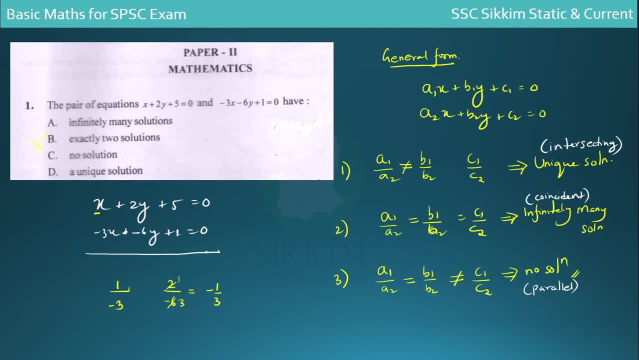 2 and 3 are equal to 6. Minus 1 by 3.. So our two ratios are equal, But look at the third. What will be the third? It will be 5 by 1.. Isn't it? 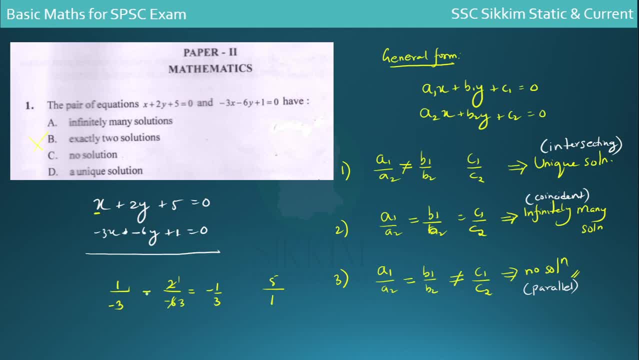 5 by 1.. So what will happen here? 1 by minus 3 equals to minus. 1 by 3 is not equal to 5 by 1.. So a1 by a2 is equal to b1 by b2i. 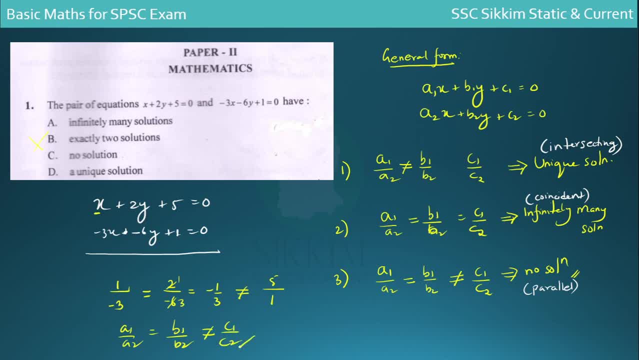 But c1 by a2 is equal to b1 by b2i, But c1 by a2 is not equal to b1 by b2i. So what will this be? What was our condition? This third condition? That is no solution. 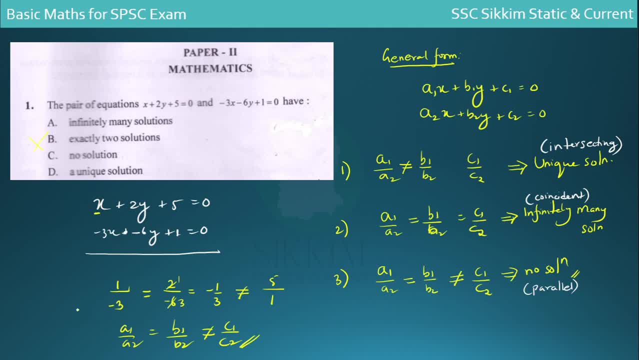 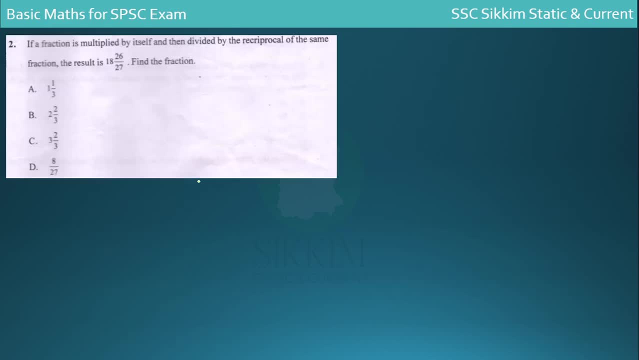 Otherwise its graph will be parallel. So option number c is the correct answer. No solution: Okay, So this was the question. Next, If a fraction is multiplied by itself and then divided by the reciprocal of the same fraction, the result is 1826 by 27.. 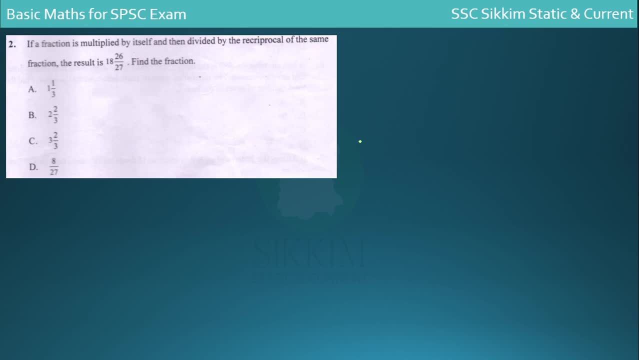 What is the fraction? I was asking an interesting question. If a fraction is multiplied by itself and then divided by the reciprocal of the same fraction, the result is 1826 by 27.. Now we don't know the fraction, So what will we do? 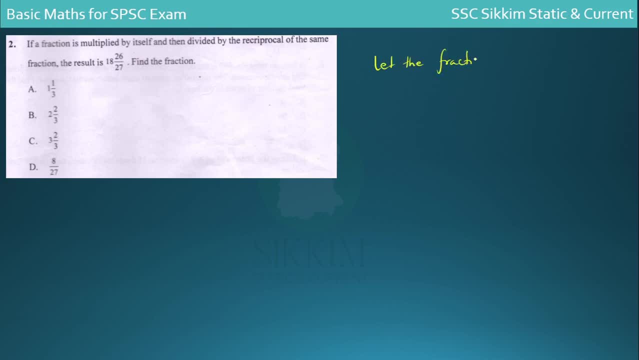 Let the fraction be. What should we do? Should we do a by b, Or should we do x by y, a by b, x by y? What do you think is easier? Let's do that. So what happens If the fraction is multiplied by itself? ie multiplied by itself? 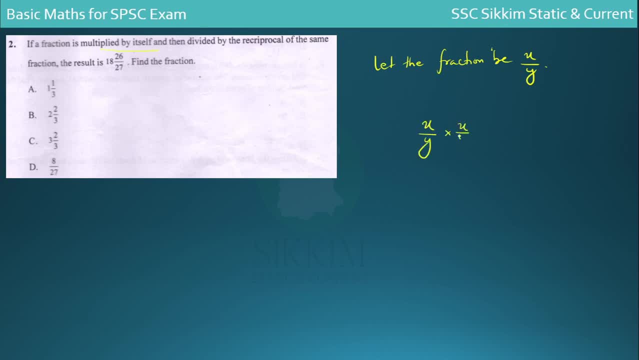 there is x by y. So let's make an example: If there is x by y' Then the x of Y is equal to No, no one more. X of y is equal to 7 x 2.. Because the الد трj is equal to 1 сz. 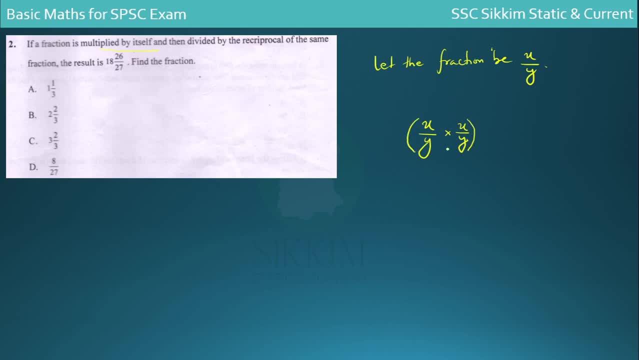 So what is the relation of x by Y with x? Well, if the fraction is divided by the reciprocal of the same fraction, then a by b, x, 2 is equal to x. I have to divide it. That fraction is equal to cons. my 2nd question. so let's divide it by 2 and start answering. 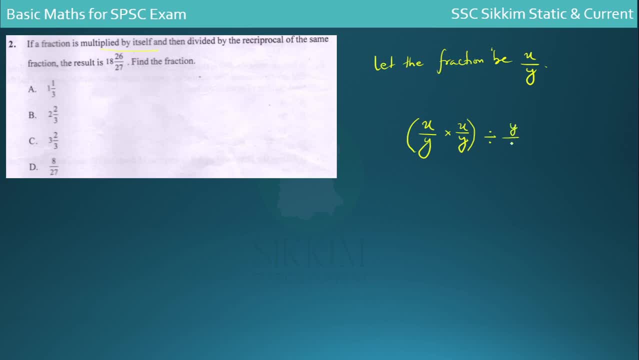 it lead by children's question in my third question, and then we can solve the problem. And what I have to do, That is it. Now let's do the first question. Let's do next question. yes, What will we do? X lady white warrior. so he so got the kids a result: kio 18, 26 by 27 io fraction. 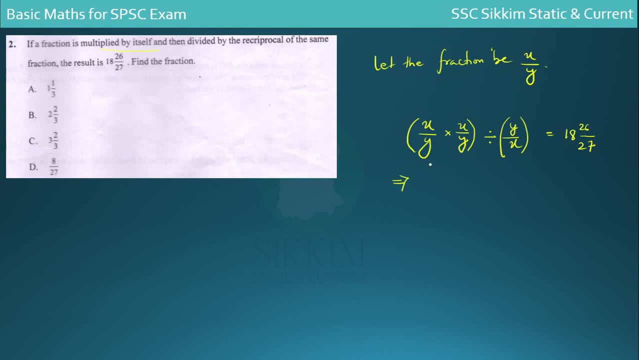 kio one of the. so this, let us see, you know, slug x by y into x by y. the capon, sir, x square by y, square on sir, okay, about divides. I double y, y, X, X card in on sand divide market. upon dinner I'll divide key on the in tunes a X math is. 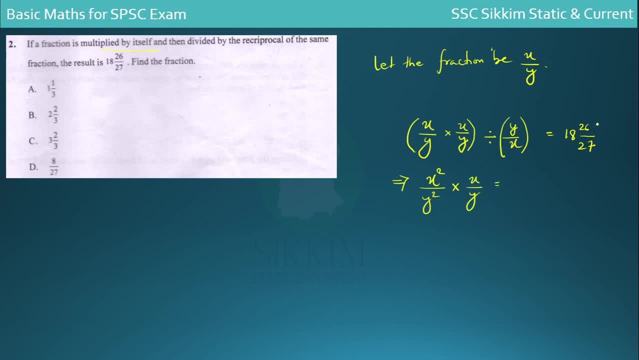 answer why? money also, and they are 27 into 18 plus 26, got the most mixed fractions. I improperly what I think he wants. a 27 into 18 gonna stay eight, sevens. a 56, 8 to the 16 solar patch, a case. so 27, so 6, 8, 2 plus 2, 4, now 486. 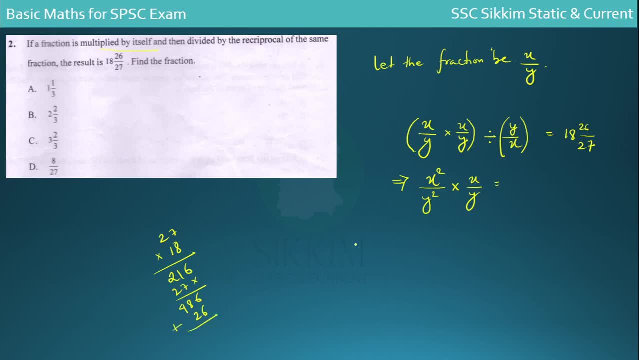 method will go to do for a 26 or no, for a no, no, mix time proper. got the kitty so he wants a 6, 6, 12. are doing the cycle a gara, so kati way 512, talaq away 27 okay. 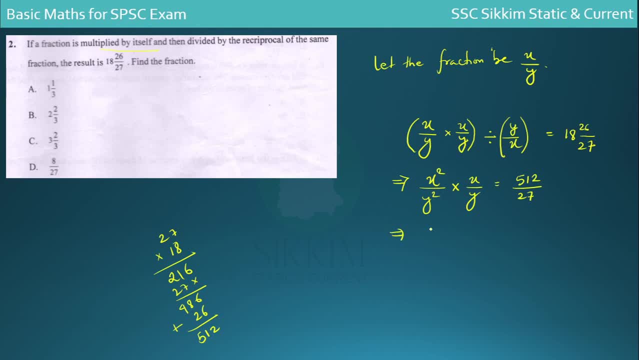 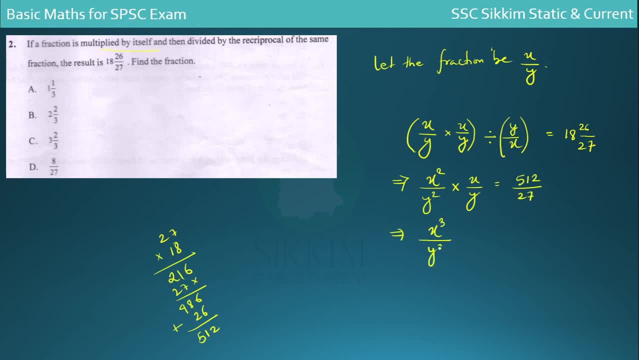 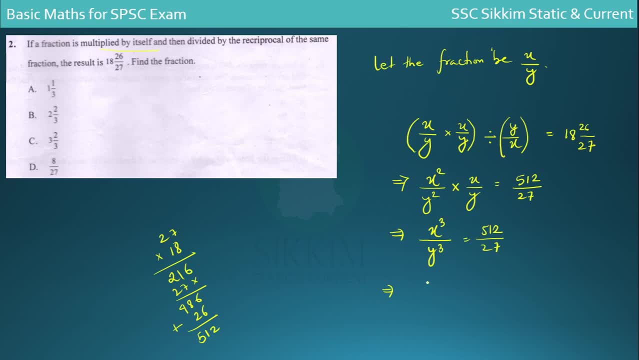 majdirak or ak mumu, ex-God buy YQ busy goes to 52 by 27 minutes. a x, y, y, ko, whole cube of the clarity, right, sir? 52 by 27, thou such a 512cido, a little cue, bunza. 27, bravo, you're cooking and say X, Y, Y, take a pyoman, the ell alignment I. 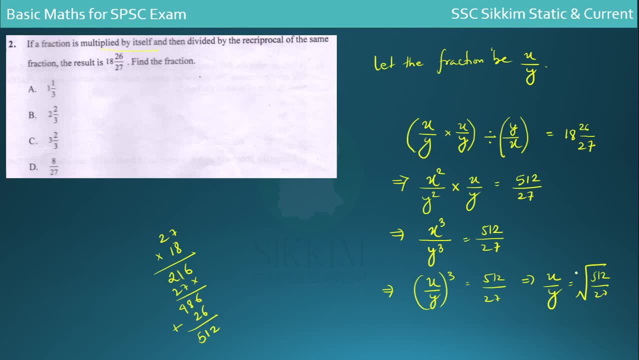 cube root of five and two by five and two by 25, kept up five hundred and six years. cube root is written as 3, so what is x by y, 512. cube root is 8. 8 into 8 into 8, 27 cube root is 3. 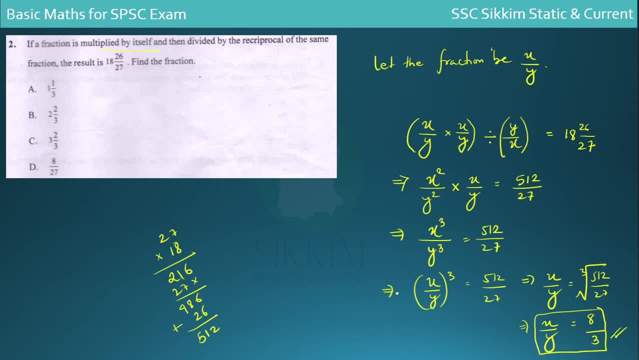 so what is the fraction at the end? 8 by 3. but we don't have 8 by 3, so what we have to do is 8 by 3. improperly convert to mixed fraction: 3 times 2 is 6. 6 times 8 is 2. 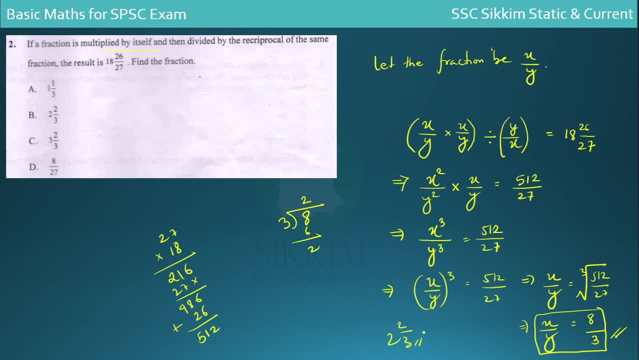 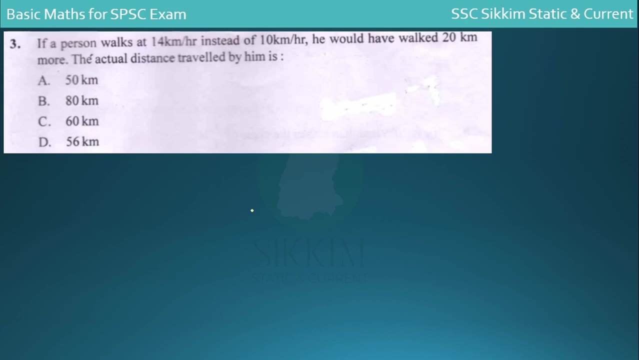 2 times 2 by 3. that is in our option, in option number b. so the correct answer is 2, 2 by 3. next, this is also my question: if a person walks at 14 km per hour instead of 10 km per hour? what is the average speed of a person walking at 14 km per hour? 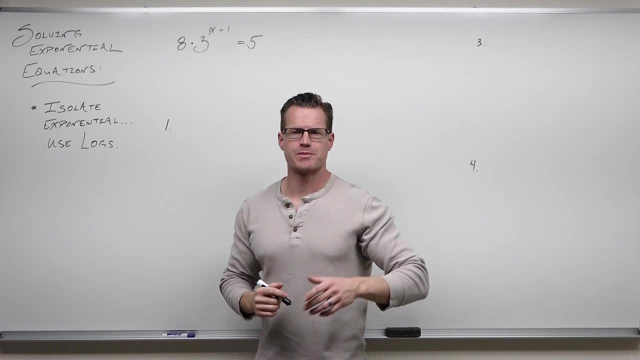 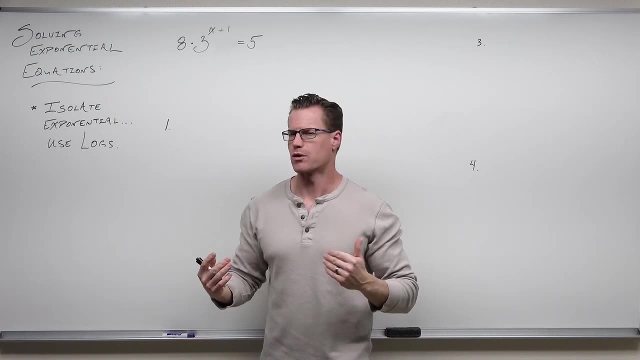 Hey there, welcome to another video. In this video we're going to solve some exponentials. So I'm going to show you four different ways to do that with a basic exponential and one way to do that with some more advanced exponentials. So we're going to talk about what in the world it 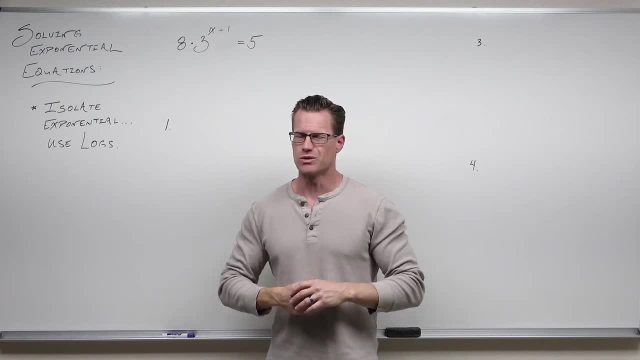 means to use a logarithm to solve an exponential without common bases. We'll discuss common bases a little bit- but I'm not going to go into this video, since we've already done that- And then I'll show you some substitution techniques to deal with some exponentials that don't look exactly.